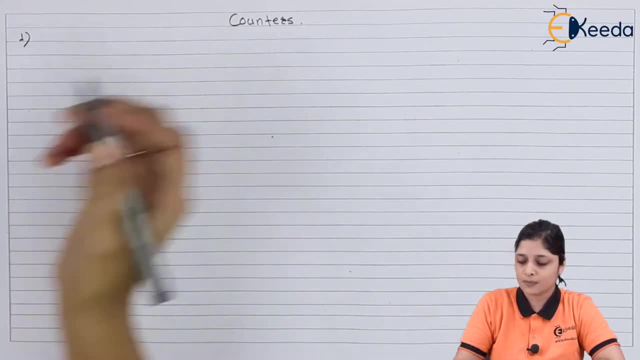 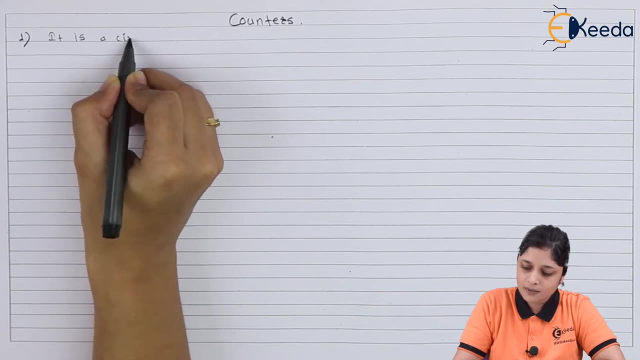 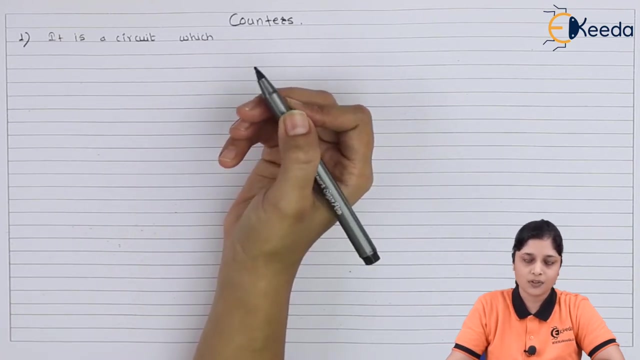 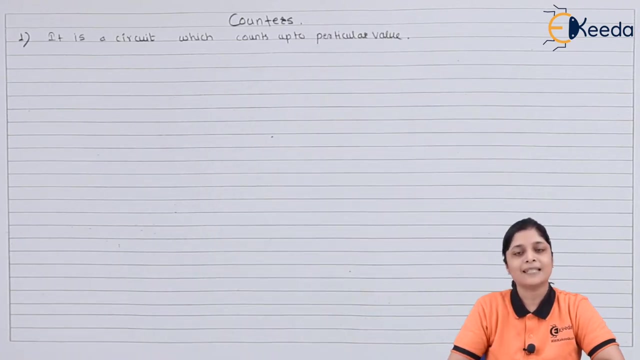 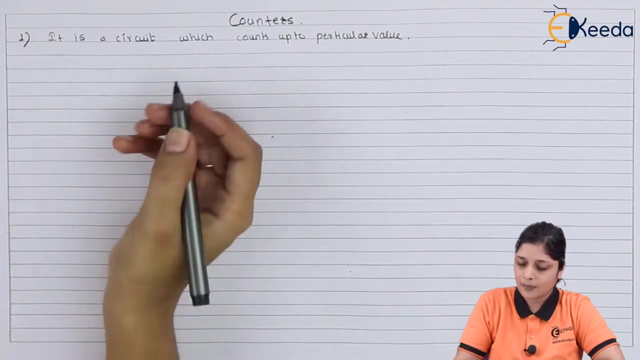 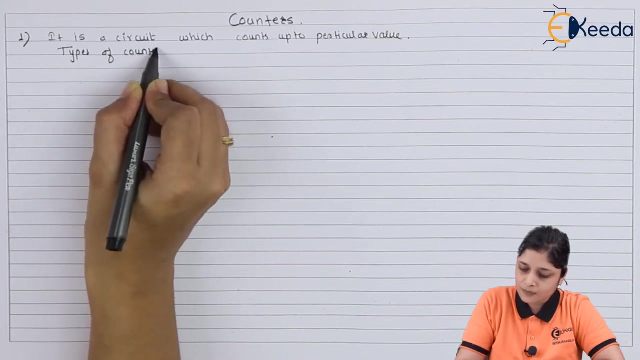 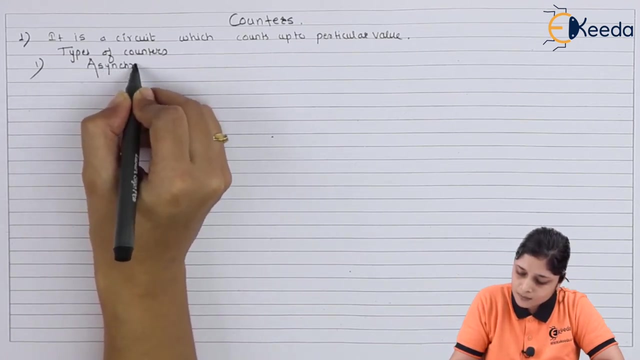 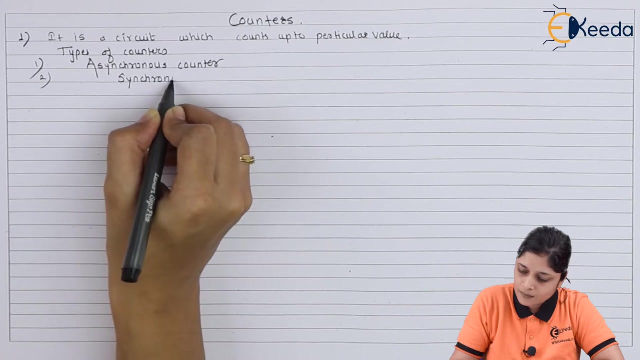 applications. So your main point is: what Counter is a circuit? It is a circuit which counts up to a particular value. Now, basically, there are two types of counters: Asynchronous counters and synchronous counters. So types of counter we have. First is what Asynchronous counter? and second we have synchronous. counter- Asynchronous counter. Asynchronous counter is also called as synchronous counter. Asynchronous counter is also called as synchronous counter. In asynchronous counter the output connected to the clock input of next flip-flops- Number of flip-flops. you have to connect it in both the counters. that is asynchronous and synchronous. The difference is of the connection. Now, in asynchronous counter, the output of first flip-flop is connected to the next clock input of the next flip-flop. And in synchronous counter, clock is applied synchronously to all the flip-flops And we can take the output. at any stage. Now further, asynchronous counter and synchronous counters are divided into three types. Let's see: So for asynchronous counter we have again three types. So for asynchronous counter we have again three types. So for asynchronous counter we have again three types. So we have again three types. 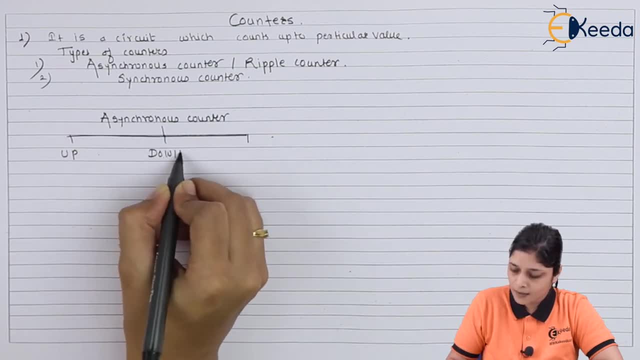 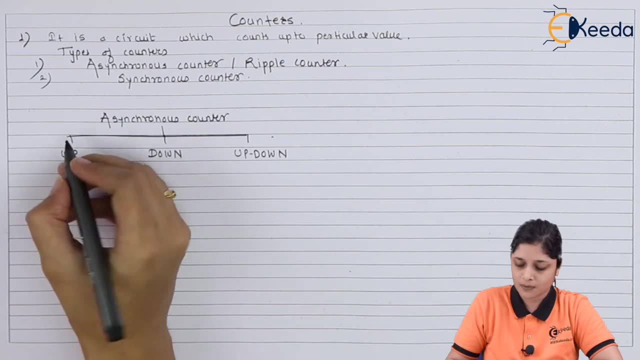 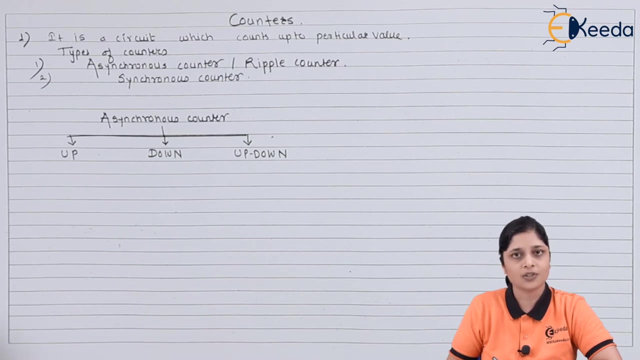 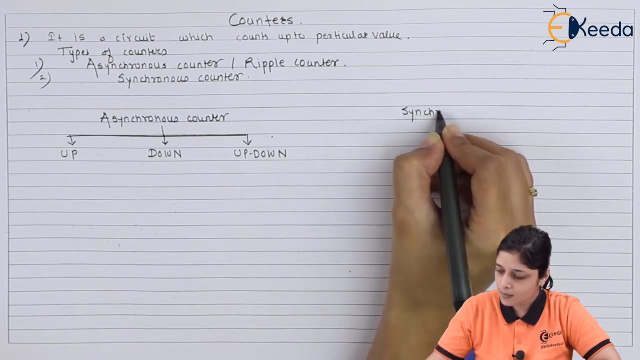 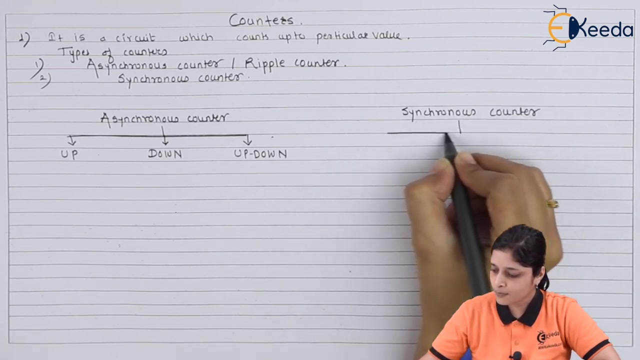 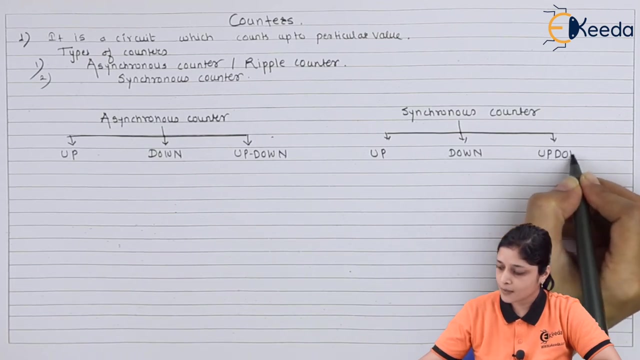 Asynchronous counter is also known as asynchronous counter, If you see the following fingers'. for synchronous counter we have again three types. the types are same: up synchronous counter, down synchronous counter and up down synchronous counter. now, at initial stage, we can start with the three bit up counter, three bit down counter, three bit of down counters and four. 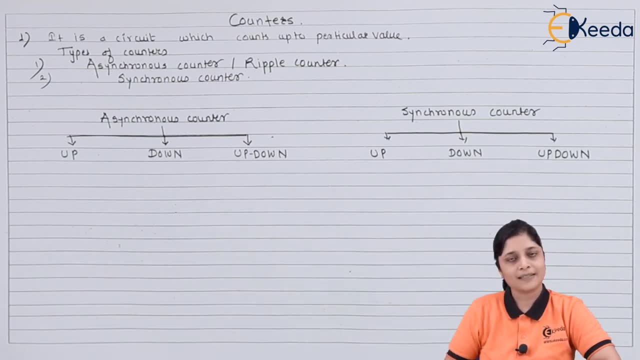 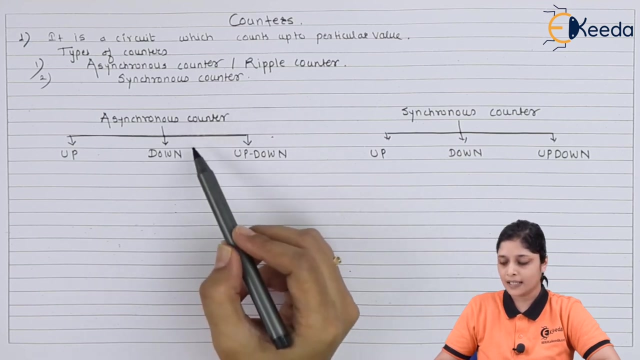 synchronous counters. also we can choose two bit synchronous counter, two bits synchronous up counter, three bits synchronous down counters. so in this way this is the bifurcation of counters, like a synchronous and synchronous. again they are divided into this three types. this is all about the concepts of six biimentoughter problema. ok, 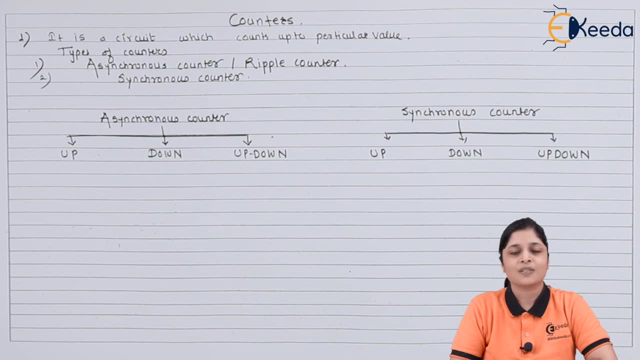 of counters. Thank you for watching this video. Stay tuned with Ikeda and subscribe to Ikeda.